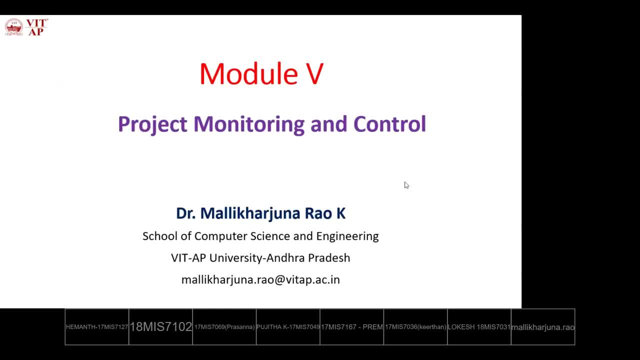 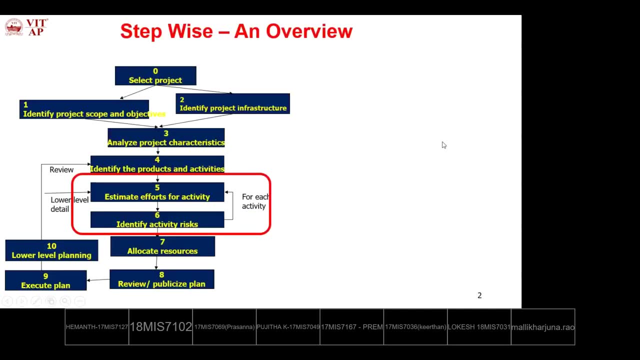 So in this video we will learn about project monitoring and control in module 5.. Before going to project monitoring and control, we will quickly review some of the topics that we discussed earlier- classes which are useful to discuss about monitoring and control. So now we are in this in this step, actually step 7.. So before going to the step 7,, 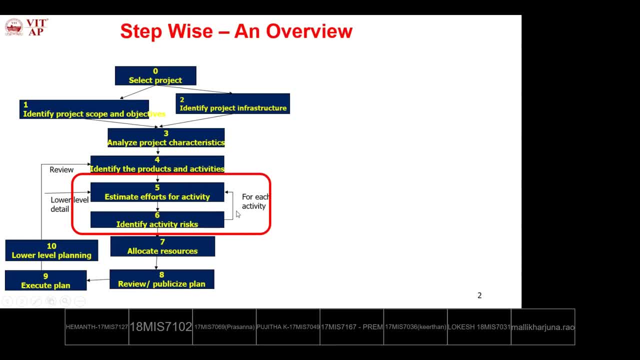 we will discuss about the step 5 and 6 quickly. So what step says? step 5 says estimate efforts, Estimating the project effort. So what do you mean? effort, Calculating how many human resources are required to develop. 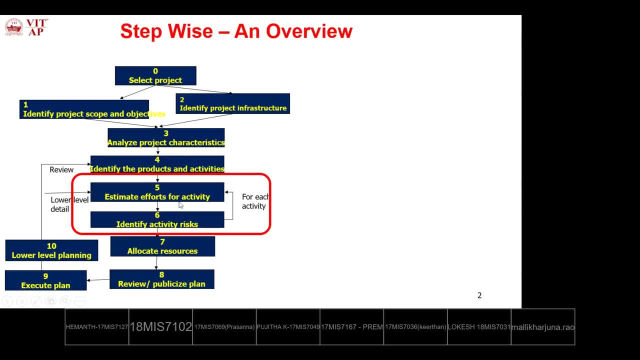 the complete project. So in order to estimate the effort of the software project development, we have different methodologies. So we will see that methodologies quickly. So the first one is lines of code. So what happens in lines of code? We are counting the number of. 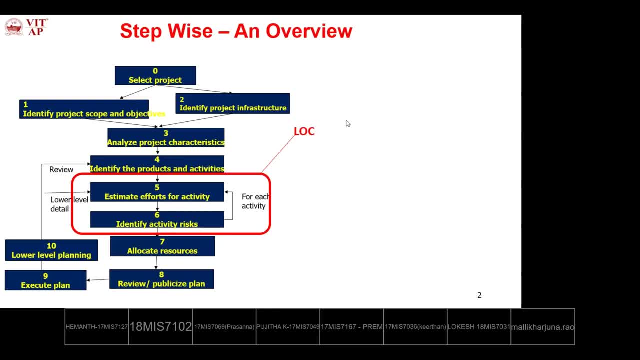 lines of code is implemented in the whole project. So initially the project is divided into various modules. So each module is divided into furtherly sub-modules, sub-modules, into various sub-sub modules, until finding the lower level elements called objects or grains. So here we are. 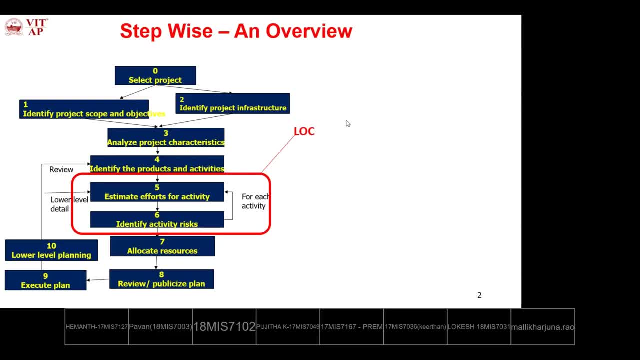 trying to identifying objects, Why objects, Why objects are playing key role in project development. So what is an object? Object is a real-world entity. Okay, object is a real-world entity. So in during project development, we are trying to identifying the various real-world entities that are existing in the project. Okay, 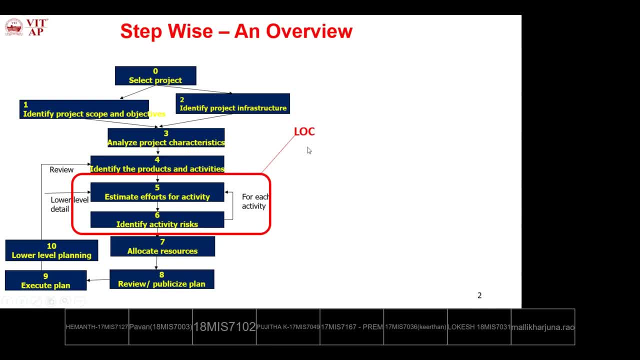 so that is a from top to bottom. Okay, After identifying these, we need to implement each and every object and the parent object, grandparent objects and great grandparent objects until finding the solution for the top chicken or the dominant, typically two or three children from the children. 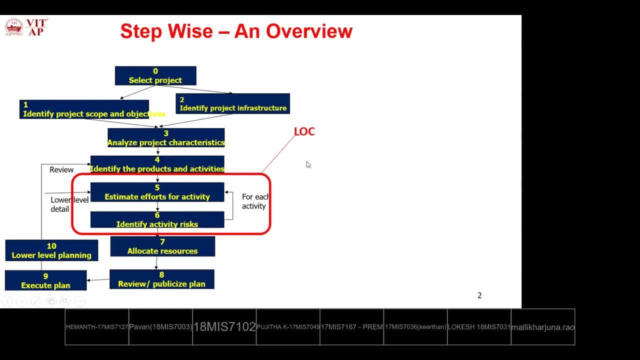 So here we have to count all the lines of code that are implemented in object parent object, grandparent object, great-grandparent objects. So that is happening in lines of code. estimation methodology counts the lines of code implemented in the whole project and estimates the effort. 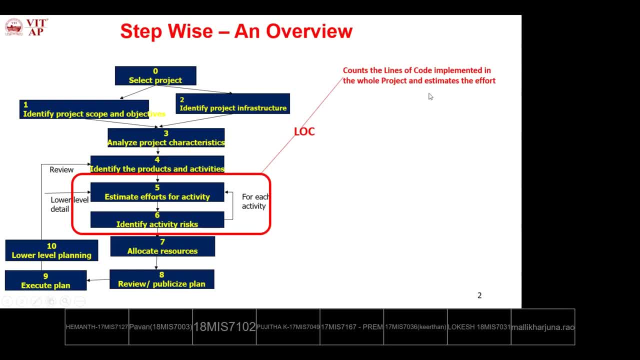 So prior to development, we will estimate. that is a planned, planned effort. So during development we are trying to estimating the effort again. So in order to deliver the product to the client by the given deadline, we are estimating. So that is simply, we are checking whether we are working according to the schedule given. 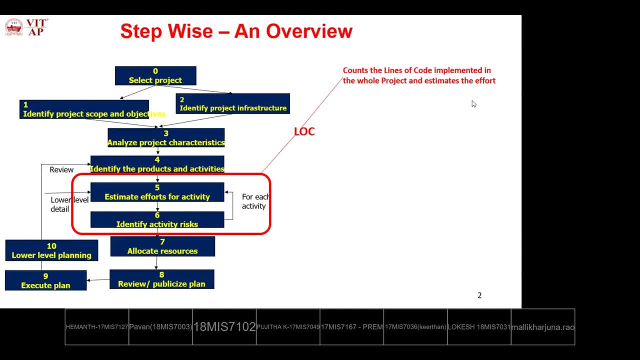 by the management or not, In this lines of code, how we, how we will estimate, We will find effort by using three techniques, that is, cost per line, total project cost and effort. Each line is estimated in terms of financially, in terms of human resources, in terms of software. 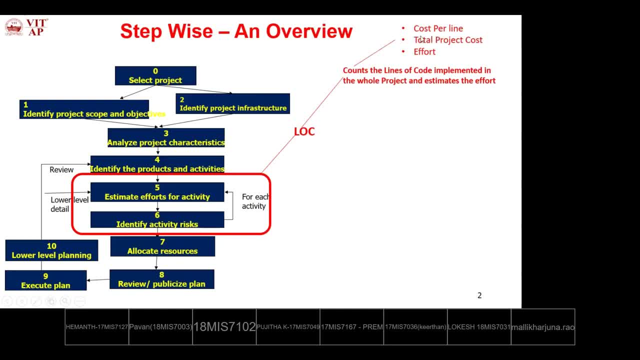 resources. in terms of hardware resources, Each line is estimated And then using this cost per line will estimate the total project cost. Okay, Here we will estimate each line in object: parent object and grandparent object, and so on. Okay, After identifying individual objects: cost per object. cost per parent object. cost per 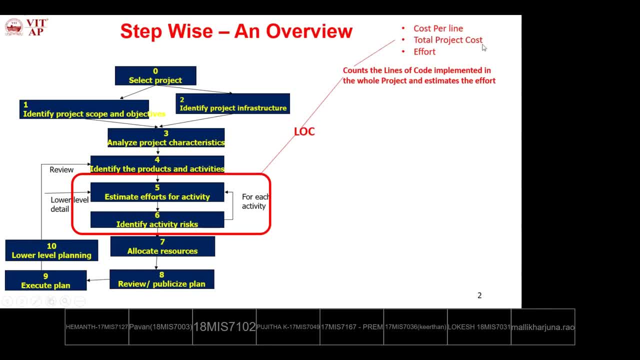 grandparent object and so on. Okay, So we will estimate the total project, that is, the cumulative project cost. Okay, After identifying this, we will estimate the effort which is useful. how many human resources are required To develop the whole project? 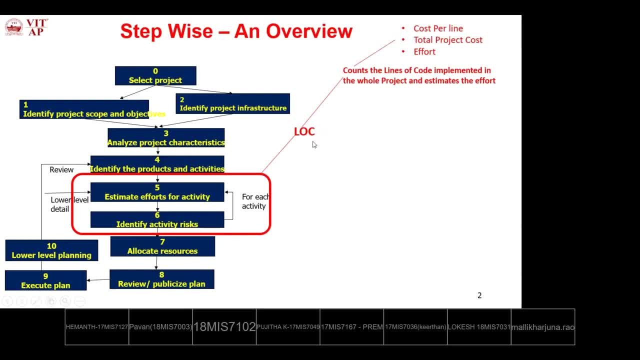 Okay, That is a happening in lines of code estimation methodology. The second method is function point. Already we are having lines of code. What is the need of function point? So if you see here lines of code, we have to estimate the cost for each line. 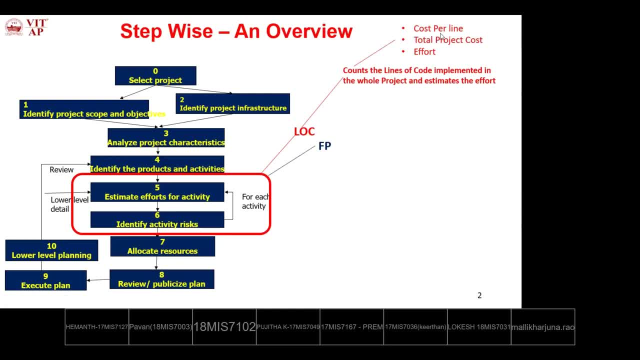 If it is a small scale project, we can estimate the cost for object and parent object and the cost per line Right and grandparent object if it is small scale project. if it is a large scale project, it's not easy to estimate all the project cost at a time- never overnight- so we have to. 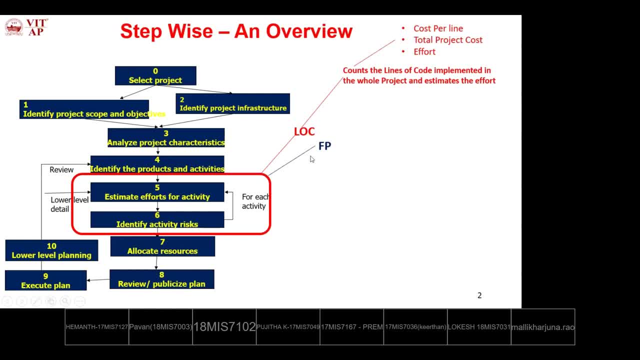 estimate the whole project cost using the other methodology called function point. okay, so what happens in function point? so here we are trying to identifying the various functionalities that we are providing through the system. so that we discussed in step one project scope and objectives. okay, so what are the various functionalities are defined in project scope? okay, so those. 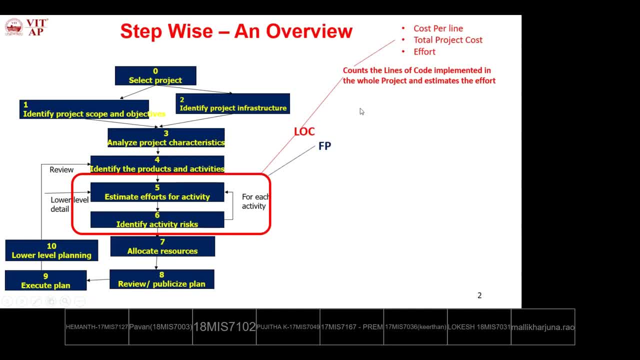 functionalities are estimated, okay, in terms of function points. in terms of function point, so counts the function points implemented in the whole project and estimates the effort, effort of each object, parent object and so on in terms of function points. okay, so how to find this functionality? okay, these functionalities are divided into, furtherly, various functional units. so, majorly, 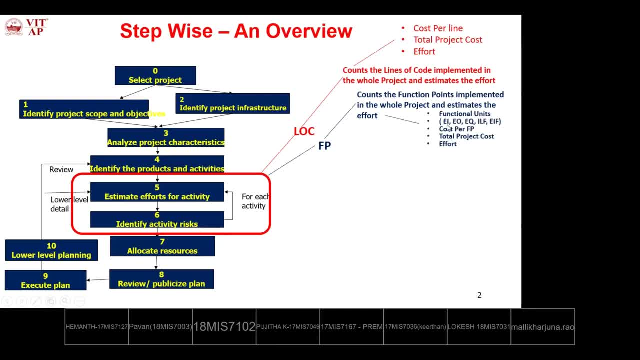 five functional units. okay, number of external inputs that we are supplying to the system. the number of external outputs that we are generating and the number of external inquiries that are made by the system internally and various internal logical files and the number of external interface files that are. 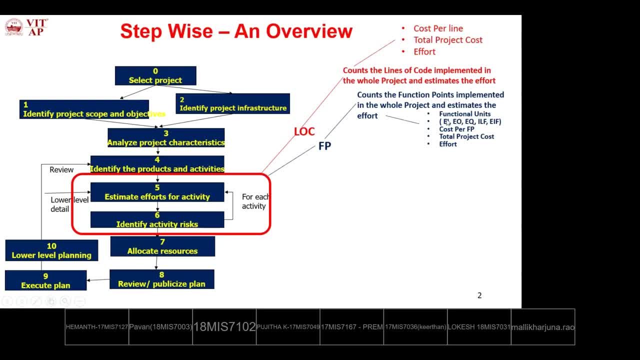 used in the project development. okay, these are the five functional units. using these functional units will calculate function point. after calculating the function point for each function point, we have to estimate the cost cost for each function point: parent function point, grandparent function point, and so on. then, using this cost for function point will estimate the. 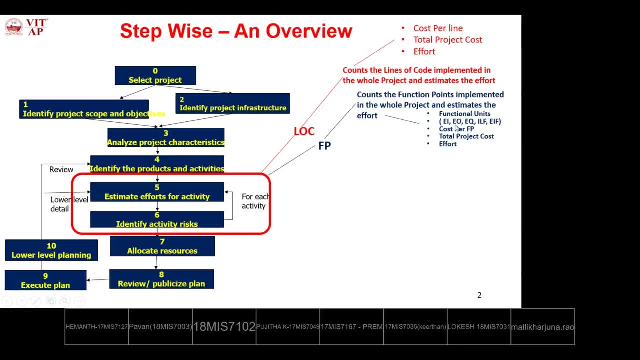 total project cost. okay, after finding the total project cost will estimate the effort. okay, so comes to this lines of code. here we are estimating for line. comes to function point. we are estimating for each function point. then the third methodology: kokomo models, constructive cost models. so these 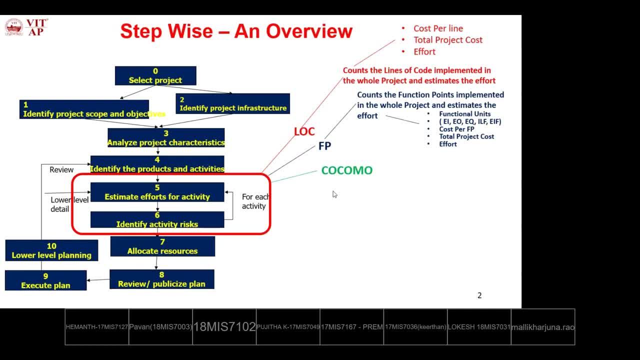 are also called as empirical estimation methodologies, so these are useful to estimate the effort. okay, so, in order to complete the project on time, okay, we, they are kokomo models are useful to estimate the effort effectively. okay, empirical estimation models are used to estimate the effort effectively. okay, so, basically this. kokomo models are divided into three types: basic kokomo model. 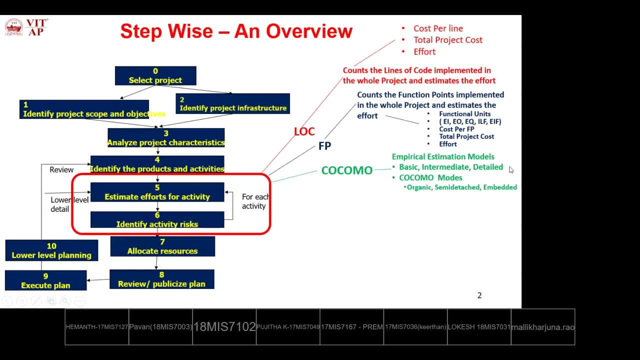 intermediate kokomo model and detailed kokomo models. so basic kokomo model is used to develop the small scale projects. Intermediate Kokomo models are used to develop the medium scale projects. detailed Kokomo models are used to develop the large scale projects. So, anyhow, these Kokomo models are used. Kokomo modes. Kokomo modes in order to estimate the 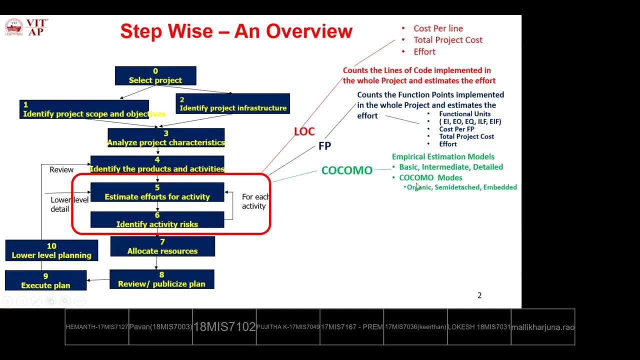 effort of the total project. So these three Kokomo modes are organic Kokomo mode, semi-detached mode, embedded mode. So we have to calculate basic, organic, basic, semi-detached, basic, embedded intermediate, organic intermediate, semi-detached intermediate, embedded, and so on depends on the situation. 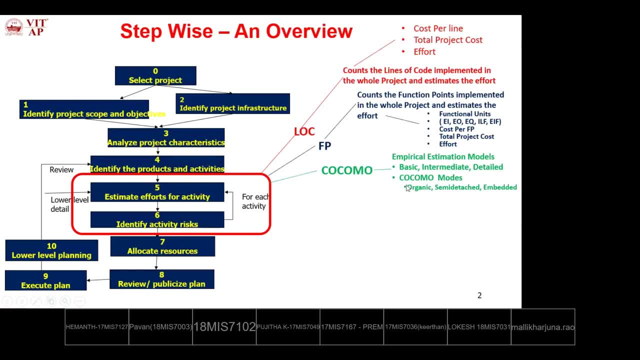 So when will we use organic Kokomo mode? depends on the size. If the size is between 2000 lines of code to 50000 lines of code, we can use organic Kokomo mode. So when will we use semi-detached mode? 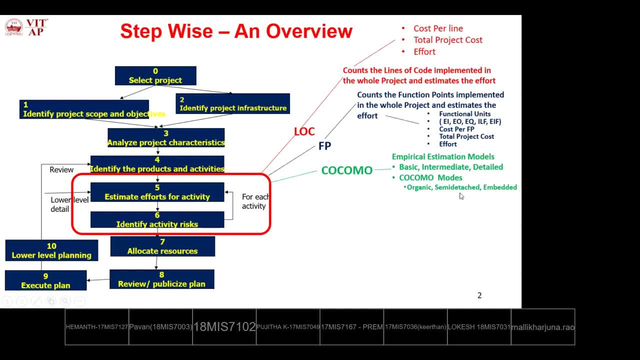 If the size is in between 50000 lines of code, we can use organic Kokomo mode. core to three lakhs lines of code will use a semi-detached mode. so other than three lakhs lines of code. so if more than three lakhs lines of code, that is a embedded kokomo mode, okay, using. 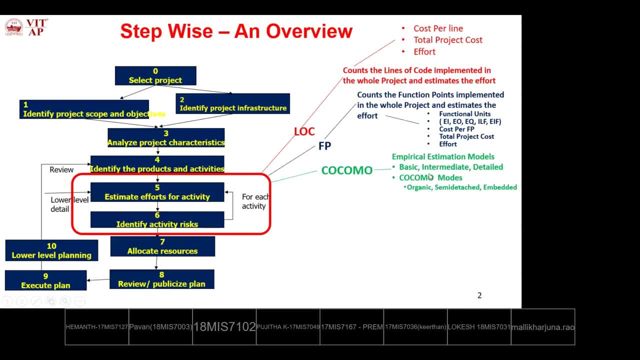 these uh pokemon models will estimate the effort of the whole project effectively. then activity planning. so in this case we are scheduling the activities. first we have to identify the various activities that are involved in the software project development of identifying the all activities. so we have to schedule. so what do you mean scheduling? so here we are starting. 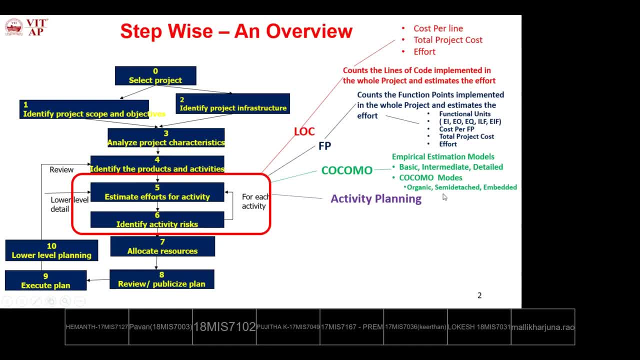 with the problem, not as a single entity. the problem is divided into smaller sub problems called modules. each module is furtherly divided into sub modules, sub modules into sub sub modules and so on. okay, so we we have to give the schedule for each uh part of this project. 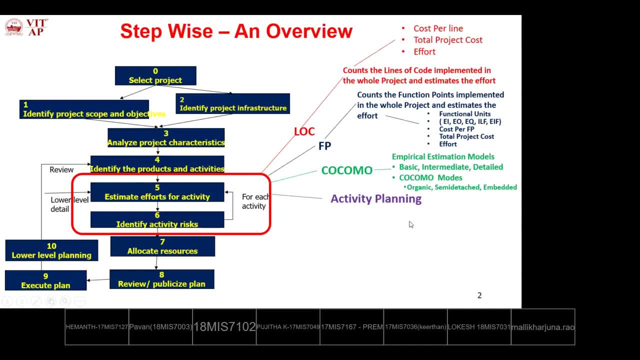 right and so on. okay, so when should we start the particular task? when should we start the particular sub task? when should we start the particular sub sub task? at the same time, when should we finish the task? uh, when should we finish the sub task that we have to schedule? 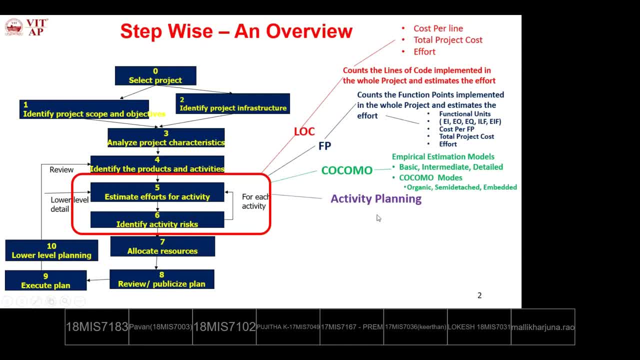 in activity planning, after scheduling the activities, we have to identify or calculate the effort of the whole project. we'll see how okay scheduling the activities, project scheduling. so, in order to schedule the project activities, so we will use three methodologies. first one is activity-based approach. second one is a product-based approach. third one is: 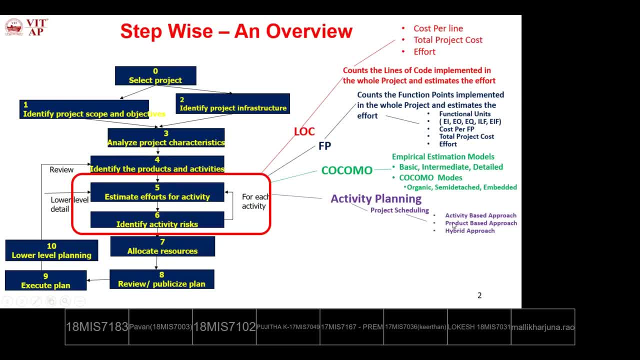 hybrid-based approach. so it comes to the first approach. activity-based approach. here we are identifying the various tasks, sub tasks and sub tasks in the starting process: the project activity, some tasks in terms of activities, okay, so these are called lower level, then product based approach. so in this case we are trying to identifying the various project products called project. 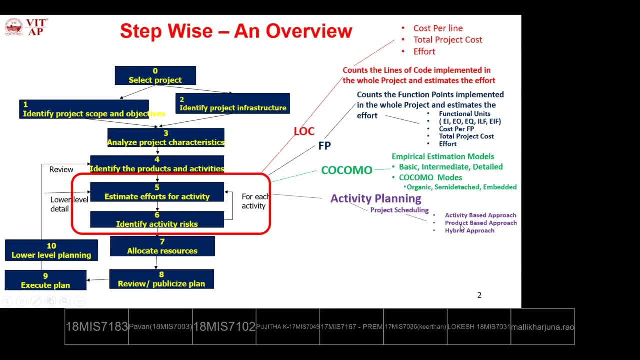 deliverables- okay, called also work products or work tasks- okay. and hybrid approach is a combination of both activity based approach and product based approach. so of identifying all the activities, we will use this approach and estimates the effort: okay, so that is when should we start? the first, the first activity, and second activity, third activity and so on? okay, same time. 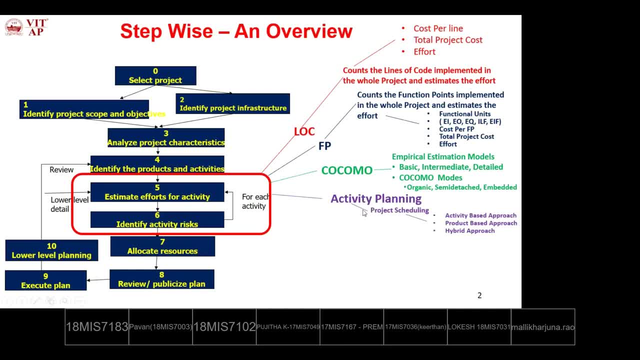 the deadlines of the activities is scheduling, project scheduling, in terms of activity planning. next, the methodology is critical part analysis and critical path method. so in activity planning the various project task tasks or activities are scheduled from day one to day n. so by, according to the deadline given by the client, we will schedule the activities. we have to finish the activities by that deadlines. 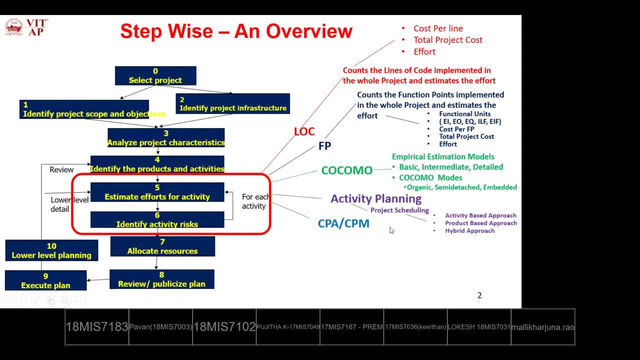 only okay. so, by any chance, if any activity or task is delayed, okay, called critical activity. okay or critical task. okay, sometimes some of the tasks are not finished by the given deadline so they take more time. those tasks are called critical tasks or critical activities. okay, so to identify those critical activities we will use critical path analysis or critical 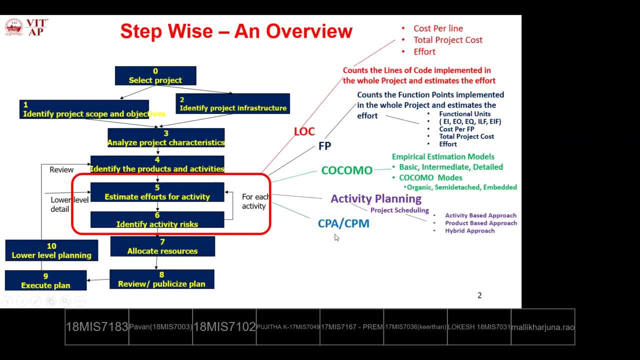 path method. okay, in order to find critical activities, we will use critical path analysis and critical path method. It finds the critical path and critical activities. okay, so these are calculated by using a deterministic time. okay, for every project product, for every module, sub module, sub sub module, and so on. 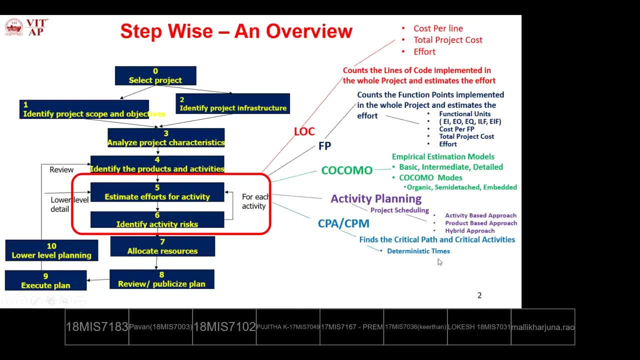 objects: okay, at the different time intervals are given, that is, the start time of the object, start time of the parent object, start time of the grandparent object, and so on. okay, or start time of the subtab: Okay, Start time of the parent task. okay, start time of the grandparent task, and so on. okay, so. 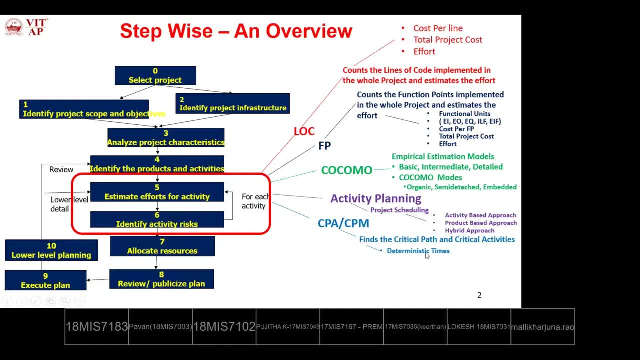 the corresponding deadline means target date to finish the activity, sub activity, sub sub activity task, sub task, sub sub task. okay, so those are called deterministic times. okay, then we will use other methodology, called PUT, in a in this step: identifying activity risks: okay. project evaluation review techniques: okay. so PUT and CPM: both are similar in a similar. 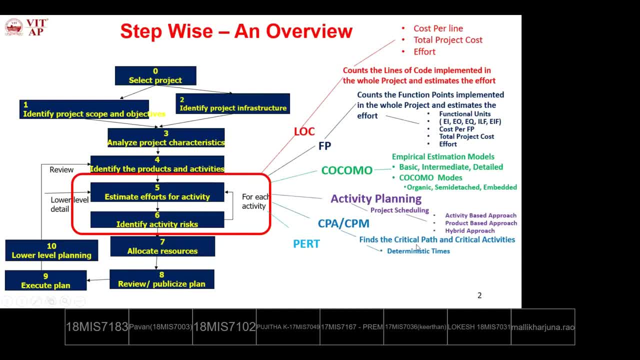 way we are trying to find the critical path. okay, so these two are differentiating one way that we will see that differentiation. okay, so PUT also used to find critical path and critical activities, so finds critical path and estimating the probability of meeting or missing target dates. okay. 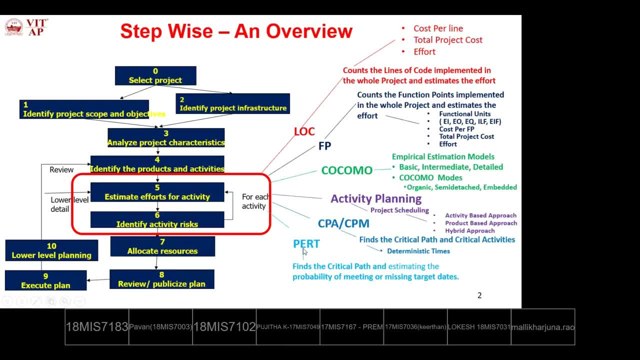 So these two methods are used to find critical path and critical activities. So PUT is used to find critical path and critical activities. So PUT and CPM are used to calculate or to identify the various critical tasks, critical activities that are existed in the project development. okay, so here every activity is. 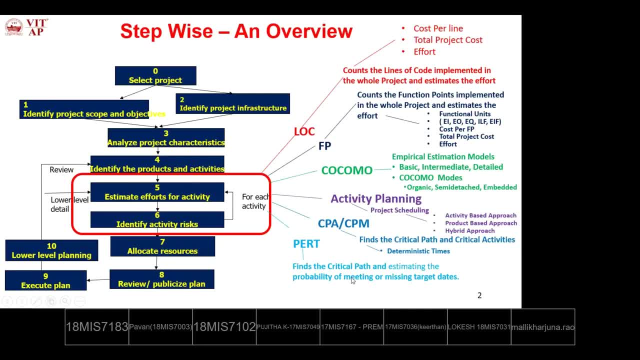 having some time intervals. those time intervals are divided into three types. in terms of non deterministic time intervals: okay. non deterministic time interval, that is optimistic, most likely and pessimistic. so optimistic is nothing but the best case that we have to start and finish. most likely, that is the average case. to start and finish, okay. pessimistic, the worst case. 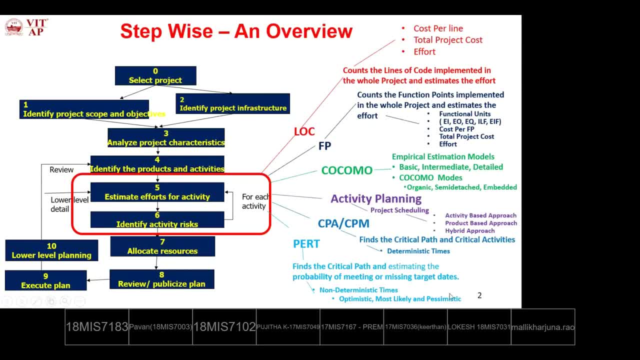 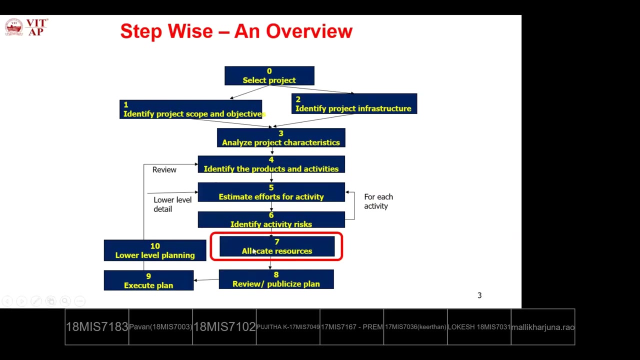 to start, to, start and finish the activities or tasks. okay, So these are the various methodologies are used to estimate the effort of the whole project. okay, So now we will learn in this video about this step- allocate resources. in coming class also, we have been discussing about this step- allocate resources. step okay, that is monitoring. 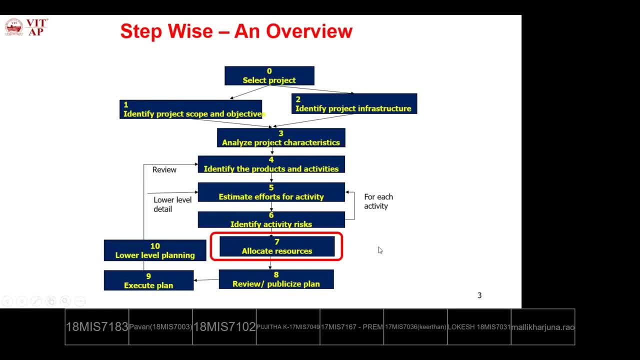 and control: monitoring the whole project and controlling the project. what is the need of controlling? okay, So generally, we are implementing the solution for a problem, not as a single unit. okay, when we collect the data, We collect the requirements from the client. those requirements are defined in terms of: 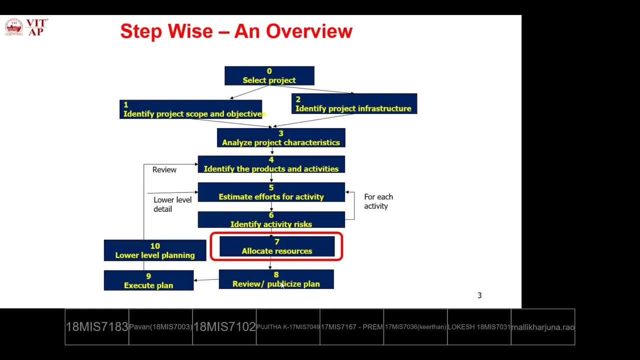 a problem. that problem is divided into various modules. each module is further divided into sub modules, sub modules into sub sub modules and so on. okay, so we have to schedule the resources. okay, so, when, when we schedule the resources, we have to keep it in mind the start. 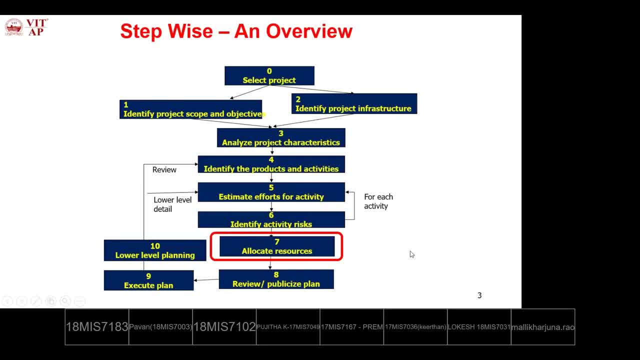 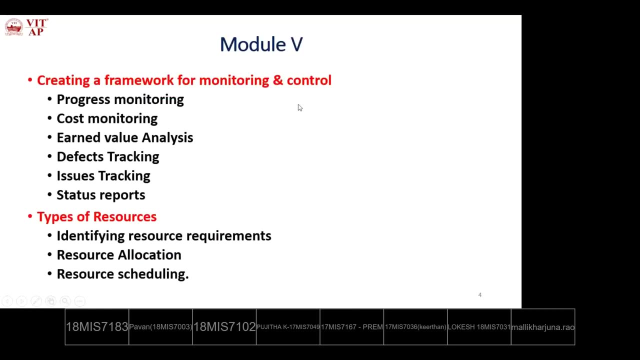 time of each task and end time of the each task. it's not a easy thing, okay. If it is a large scale project, it's a very typical thing. so, in order to maintain that, we will learn monitoring and control. okay, so creating a framework so to monitor and 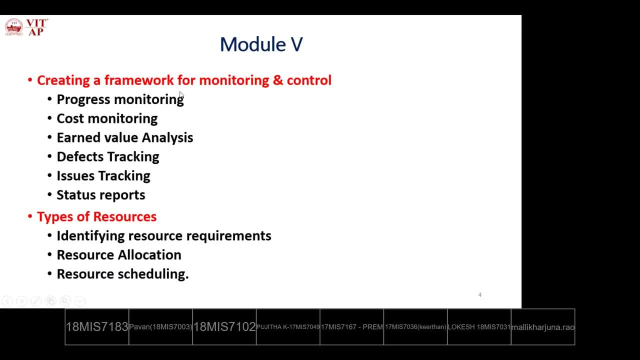 control the whole project. we will create a framework. that is the first concept that we are going to learning in this video. okay, so as part of creating framework, we will monitor the progress- Progress of what? progress of project, progress of modules, progress of sub modules, progress of sub sub modules, and so on. the same time, cost: cost of the whole project, cost of the 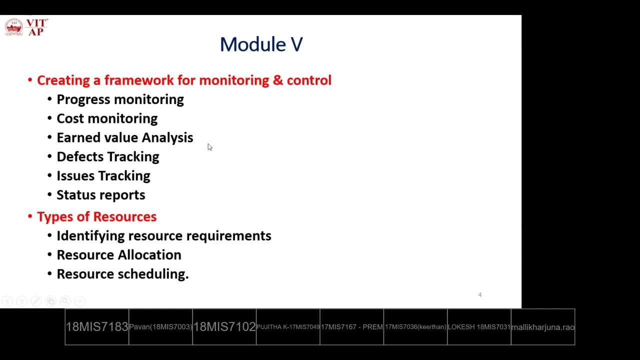 modules, cost of the sub modules and so on. okay, earned value analysis. as part of the software project development, we will estimate end value and, obviously, the returns on investment ROI. okay, You will see that in coming days, In coming classes. next, defects tracking: okay, are there any defects are existed during project? 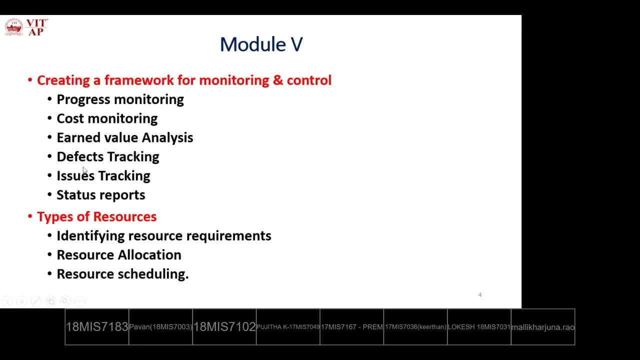 development, okay. identifying the defects and tracking: so this already we discussed in previous classes in risk analysis, and then issues: tracking of identifying the issues: okay, so we will track that issues. okay, when the issue was generated, when it is resolved, all those things are need to maintain. 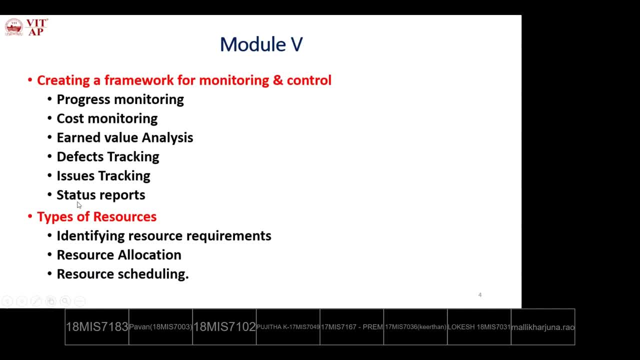 Okay, Finally, preparing a report on all the project products or project deliverables: status reports, report of project, report of modules, report of sub modules, report of sub sub modules, and so on, until for objects. okay, there is a first part: creating a framework for monitoring and. 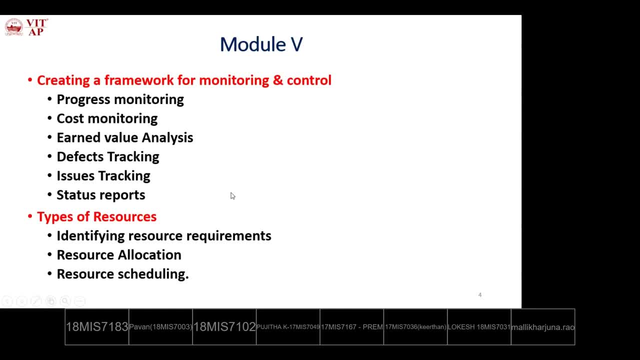 control. and the second part, types of resources. in this case we are trying to identify the various resources as per the problem definition. okay, so here resources are nothing but the various human resources are required and the various software resources are required, the various hardware resources are required and the various other environmental factors that 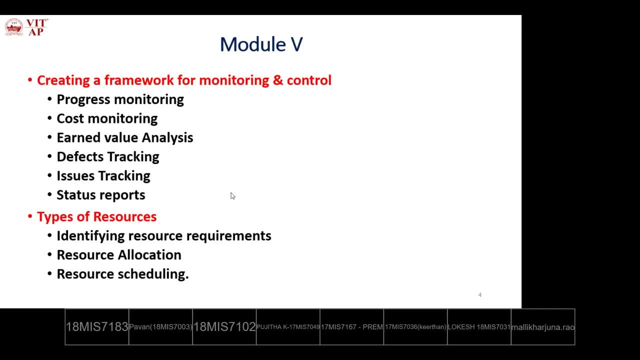 are required to develop the project. okay, that we are identifying, after identifying the resources, allocating the resources. so what is the need to allocating the resources? we can allot the resources for the project. okay, what do you mean project? the project is divided into modules, modules, sub modules and so on. okay, so we have to allot the resources. how many? 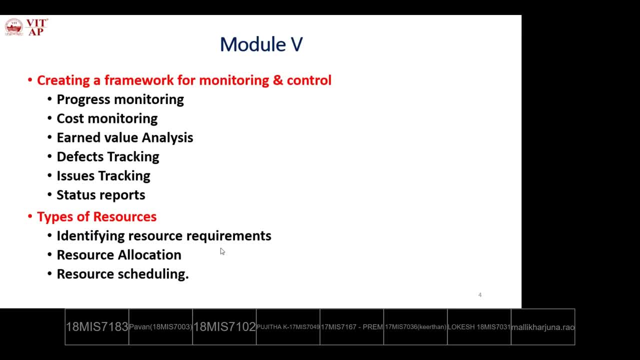 human resources are required to develop the project at the same time module, same time sub modules, and so on. okay, that we are allocating. so how? how could we allocate using resource scheduling? okay, so scheduling the resources: how many human resources, sub modules, and so on. okay, mineral services are required for to develop, subtasks to develop, task to develop. 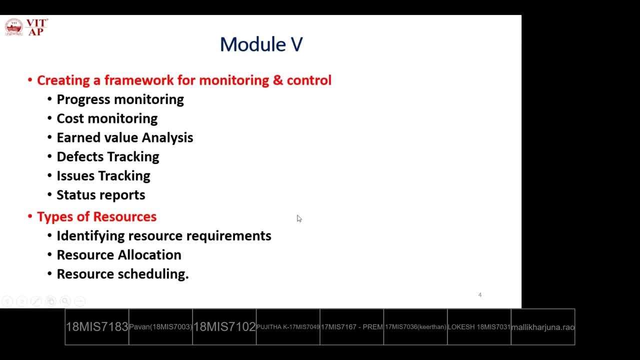 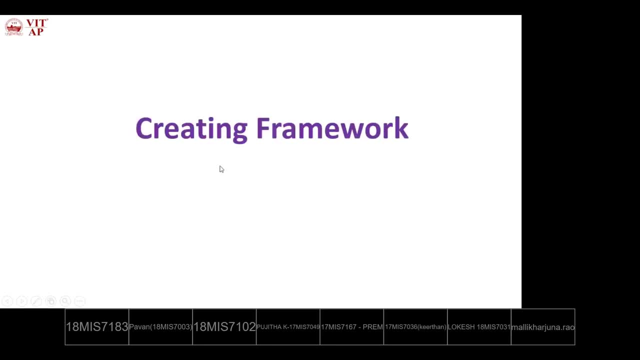 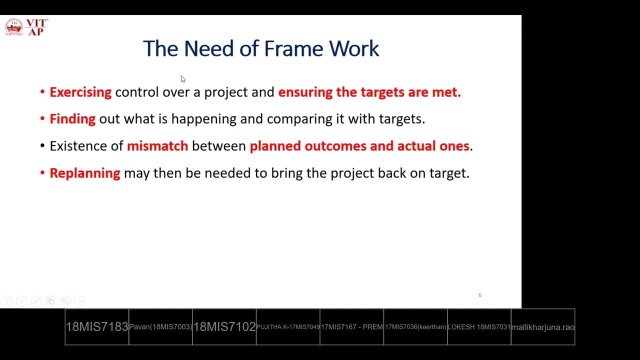 a final solution for the problem. okay, we'll see in this session, creating a framework, okay, so what is the need of framework? in order to monitoring and control the whole project, the whole project, we need a frame work. so this, very this framework is useful, excellent. so remember, this framework is used for sample. 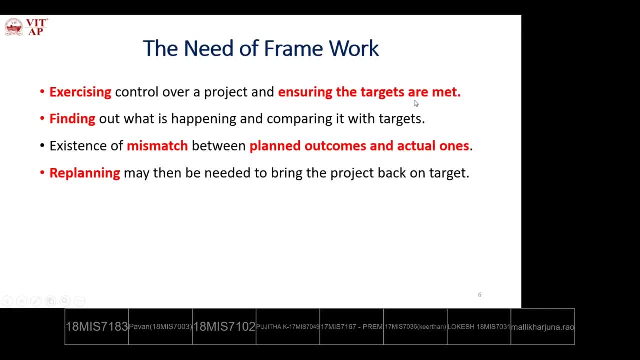 exercising control over a project and ensuring the targets are met. okay, so in project development, the project is divided into modules, module into sub modules and so on. okay, every sub module is having the start date and end date. every module is having the start date and end date. so, by the 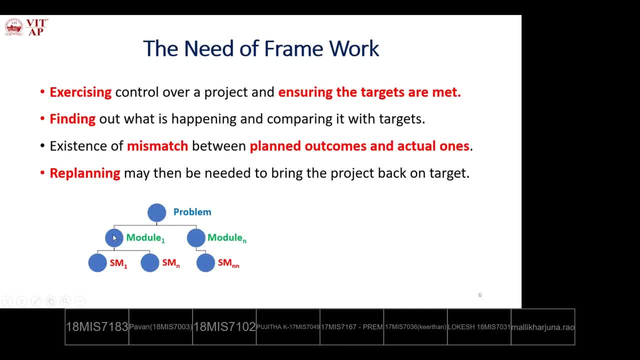 start date we have to start the activity and by the end date we have to close, finish the activity, so that we are ensuring whether targets are meeting or not. that is nothing, but whether we are following the schedule that is given by the management. okay, that we are ensuring this framework. 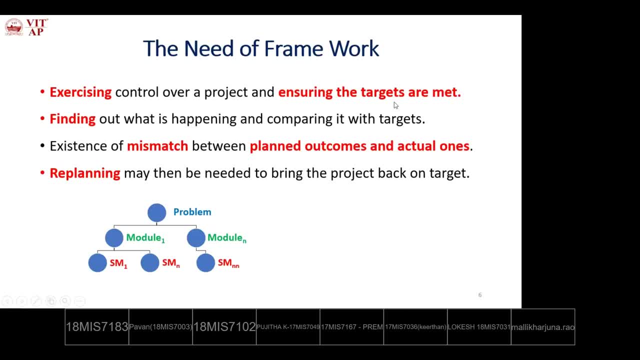 is ensuring the whether targets are meeting or not. at the same time, we are checking, uh, are the requirements are meeting or not that are defined by the client and refined by the management? okay, then framework is also useful of what is happening and comparing it with the targets. okay, so, by any chance, if any activity is, 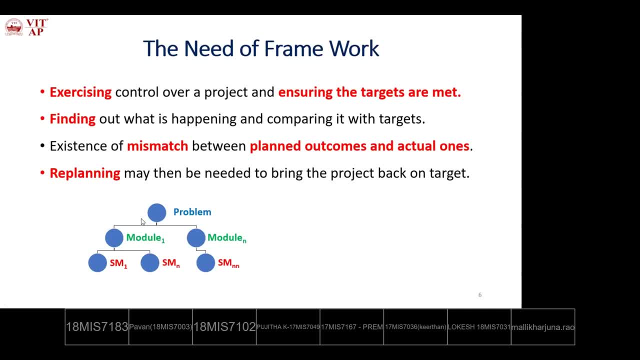 delayed: okay, in order to finish the project: okay, if any activity takes more time than the planned time. called critical activities: okay. finding the critical activities: okay, if any activity takes more time than the planned time. identifying those activities: okay. we are always checking whether we are working according with. 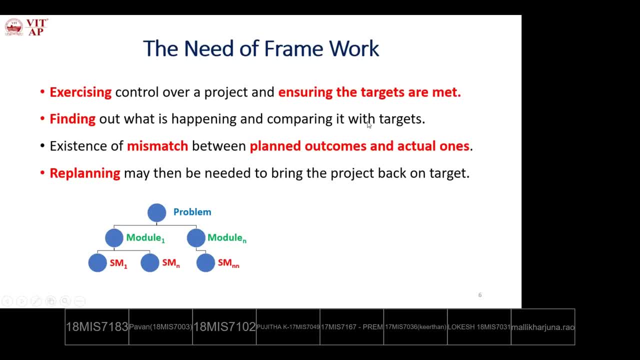 the target dates or not. okay, so, while checking if any mismatch is existed- existence of mismatch between planned outcome and actual ones. so here we are checking. what do you mean? planned outcome, so prior to development, will estimate the effort, cost, quality, etc. etc. are defined. so what is the effort defined prior to development? what is the effort that we are applying on current? 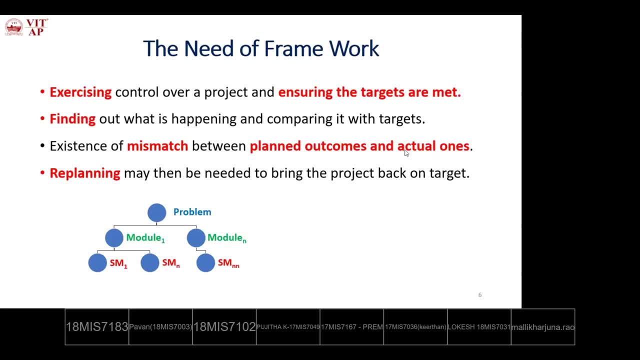 project: okay, whether matching or not. and cost: what is the cost estimated prior to the development? what is the amount that we spent on that day up to that date? okay, at the same time, quality: what is the quality is defined earlier. are we achieving the same quality or not? like this way. 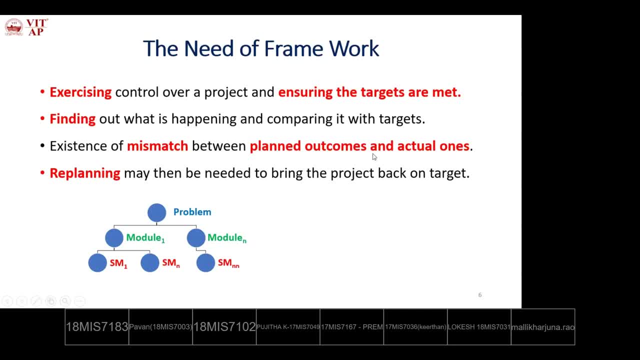 these parameters that we discussed in regular classes- functionality, usability, reliability, performance, stability, scalability, optimality, adaptability, etc. etc. are all are meeting, are not according to the schedule or not okay? R means all the project products are meeting the targets. are not okay if any mismatches existed. if the mismatch is low: okay, so we won't bother about. 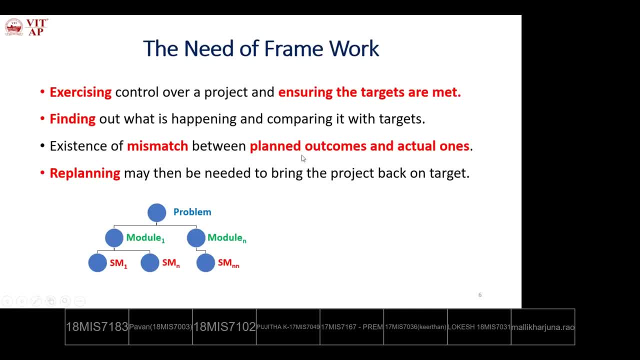 it. if the mismatch is high means if there is a lot of difference, if the gap is more, we need to replan the activities. replanning may then be needed to bring the project target. okay, replan. we need to replan all the project products. okay, so at top level you are having high level data. it is called 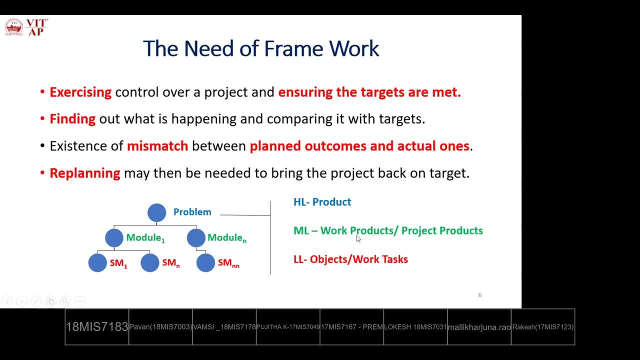 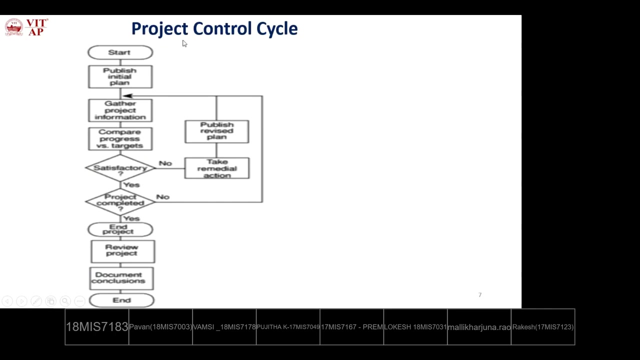 product description. in the intermediate level, you are having middle level work products or project projects. in the lower level, you are having objects or work tasks. so this is the need of framework. okay, so during project development, to monitor and control all the project products and work tasks, we need a framework now, project control cycle, in order to control the whole project. 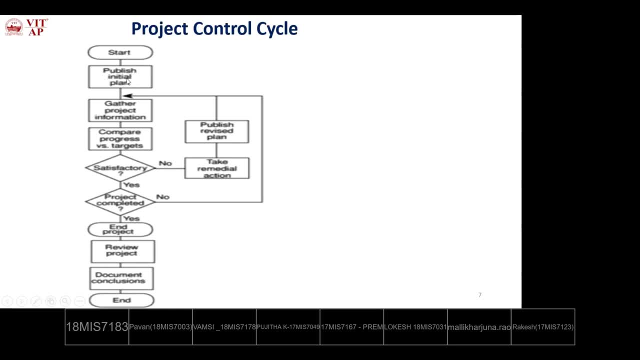 okay, so the we'll start the project. publish initial plan, that is, collecting the requirements from the client for the whole problem. after collecting the requirements, refine it and collects the requirements as per the industry need and satisfying the user or client- okay. gather project information according to the industry need and users perspective- okay, and then start. 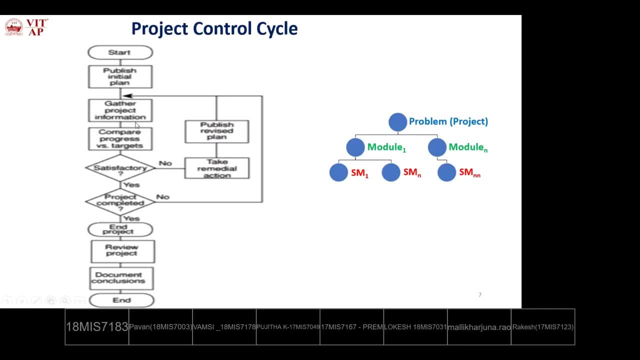 implementation and proceed towards finishing the project. okay, while finishing the project, compare progress versus targets. so, as we discussed earlier, every sub module, every sub sub module and module are having the target dates. so what? even target dates? the time that we have to start the particular sub module, the start. 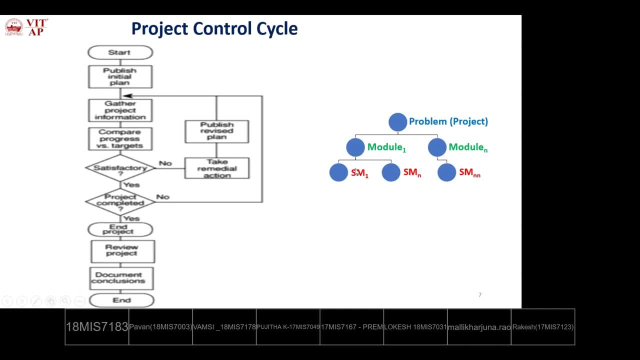 time of this module sub module and end time of this sub module. okay, so, like this way for all project products, some deadlines are given. so those deadlines are meeting or not. the same time, the various parameters- functionality, usability, reliability, performance, stability, subtraction parameters- are meeting or not in terms of sub. 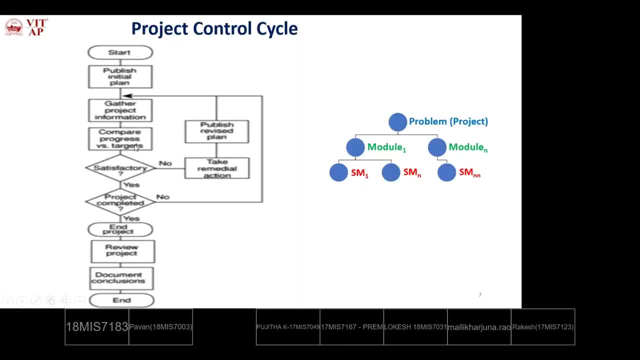 modules and modules and so on. okay, that we are checking here. if it is satisfied, will continue. otherwise take the remedial action. so that is, which, which object, which parent object, which grandparent object or which work task or which subtask is not satisfying, identifying those activities or project products, and plan the alternate solution called remedial action. okay. 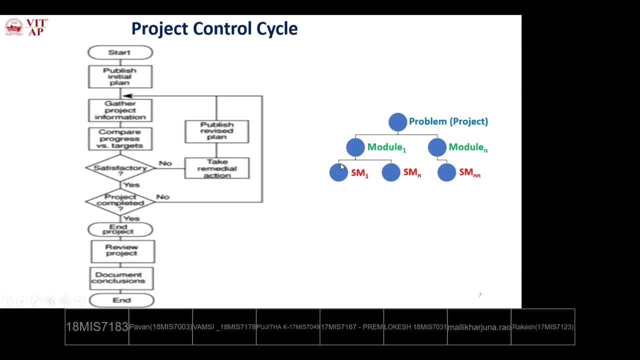 plan the alternate solution for the user. so what are these? these are what called critical activities. okay, identify the alternate solution for critical activities. so what about critical activity? an activity takes more time than the planned time or scheduled time. okay, is what called critical activity? okay, if any critical activity is existed in the project development, it shows the impact on. 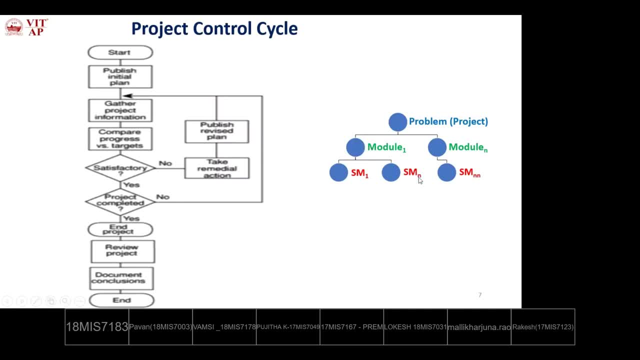 the remaining depending activities, for example, if you take this, so the, it's a part of this module. okay, so for this formula, the deadler, the time is given, 10 days, assume the case. okay, so this 10 days is split into sub module 1 and sub module 2, for your understanding sake. so it is for this: five days are. 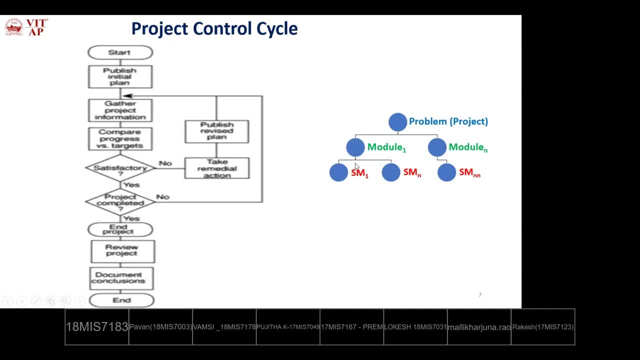 five days are given, okay. so if it takes seven days, what happens? so it has to. this model has to wait until it finishes. okay, if both are parallel activities, no problem. okay, both are not parallel activities, so nothing. but if it is depending on this critical activity, if it depends on this, so when it will start? 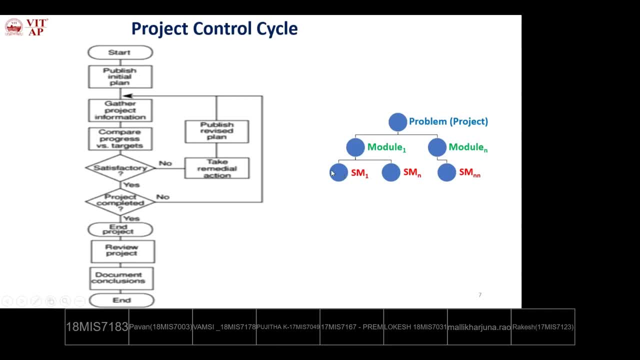 whenever it finishes. okay, if it takes more than the planned. actually, five days are allocated to to this task to finish, but it takes two more days extra. okay, what happens? we need to finish this task in the remaining time. what is the remaining time? three days. okay, if it takes more than that, okay, actually it. 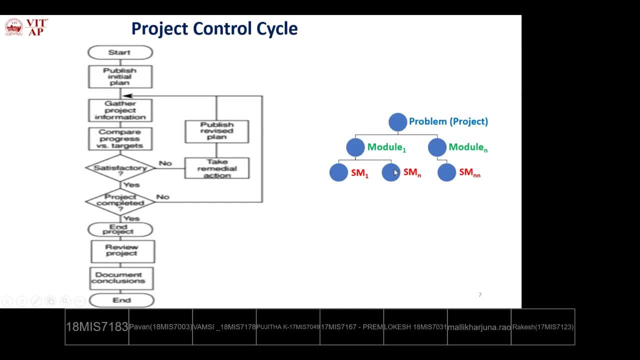 requires five days, but we left with the three days. okay, three days are not sufficient. what we have to do, it takes two more days. so what happens? so it will be delivered lately. so they are what called critical activities plan, the alternate solution for this kind of scenarios. okay, and publish the revised. 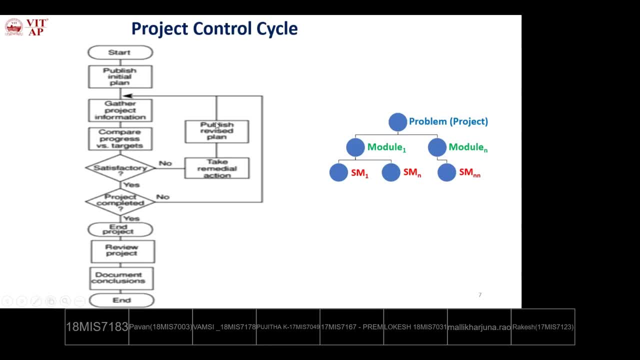 plan, the alternate plan, okay, and get approved with the client-hand management and continue the process like a cyclic. okay if it is satisfied. okay, so all are working according to schedule and finishing the according to the schedule. okay, now need to check whether project is completed or not. okay, so what do you mean? project this? okay, whether. 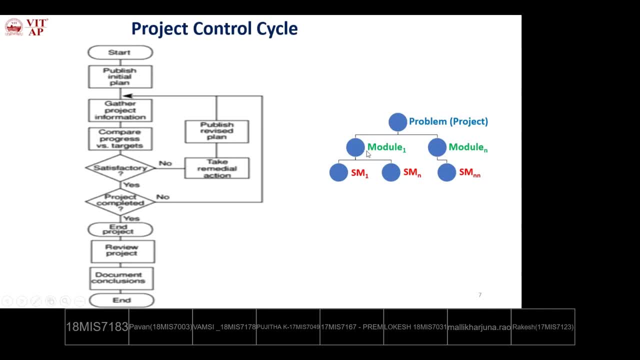 if any module is finished, we need to check whether the module is finished or the whole project is finished. so if someone says that my job is finished, okay. for example, person a allotted sm1 submodule one. so if the person's one says my job is finished means we need to check whether 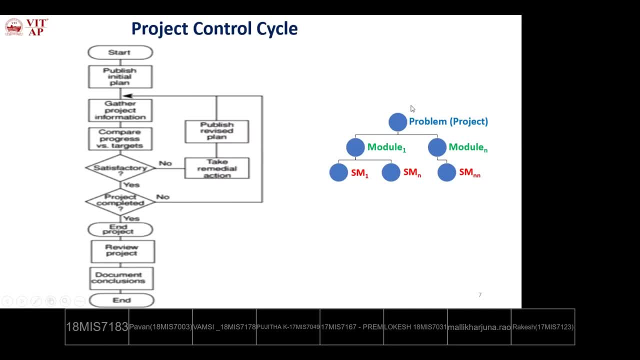 it's: uh, his job only finished. all or the whole project is finished now. his job means sub module. one solution is completed, it's a part of module, so we need to finish this. so when will we finish this? whenever we find solution for all its child problems, for all these? 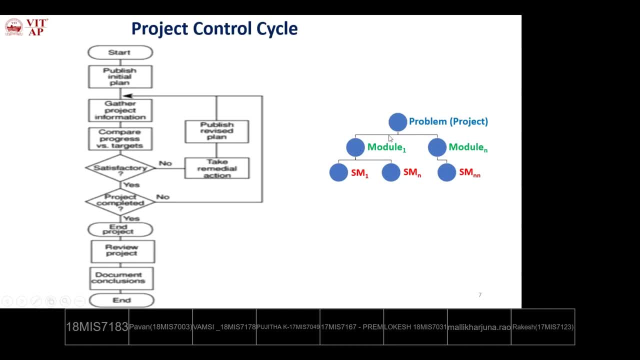 okay, then we'll get the solution for this. so when will we find solution for this? whenever you find solution for all its tails for this. okay, then only you will get the solution. okay, that we have to check whether the particular task is completed, the whole project is completed, that we have to check okay here. so if it is a task is completed will continue. 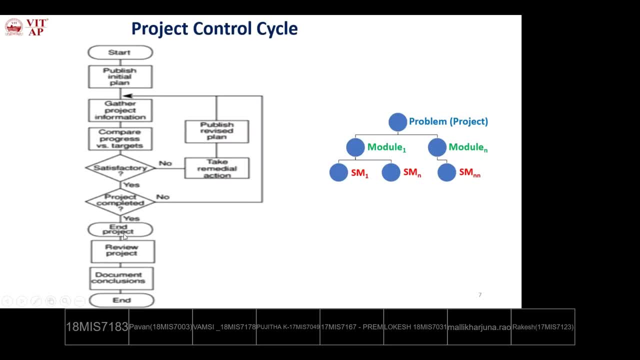 the process, if the project is completed, will end the project and reviews the project. so what you mean reviewing here? so here, reviewing the quality of the project. so what is the defined quality? is the quality is achieved or not? okay, so that we are reviewing and, at the same time, what are? 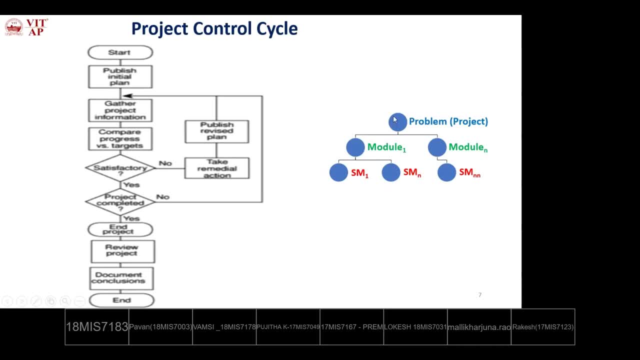 the functionalities are defined or all the functionalities are implemented or not. what is the performance issue? issues are defined or all the performance issues are addressed or not. that we are checking. once it is accepted by the client, we need to document the whole solution and the project. so this is for the whole project. 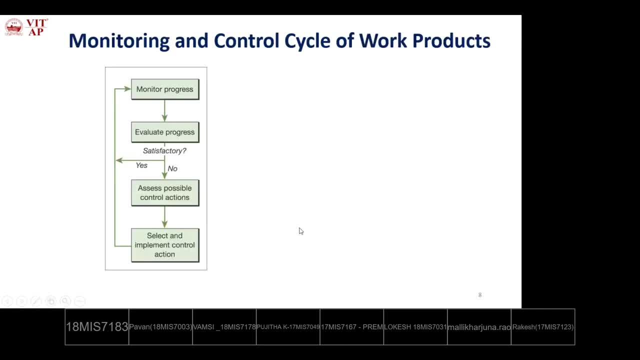 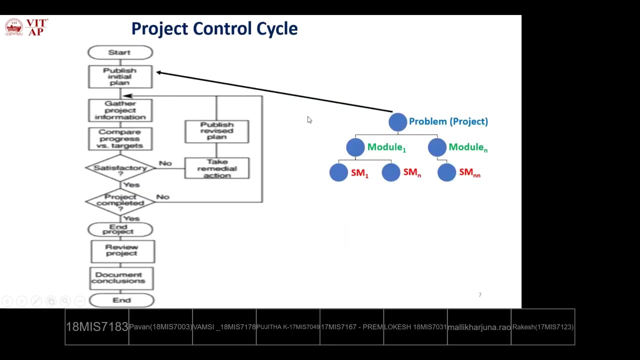 this is for the whole project, similarly for every project: deliverables. so what do you mean deliverable? so this is what called project product or project deliverable. so initially, the problem called project description is divided into modules, modules into sub modules, sub modules into sub sub models and so on. okay, so when you so, in the previous case we evaluated for the whole project. 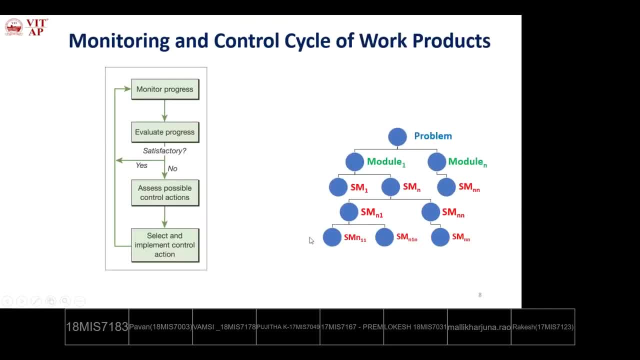 now, in this case, we will evaluate for the project deliverables that are, intermediate project products. okay, monitoring the progress of sub sub module, same way, sub module, same way, other sub modules and so on. okay, like this way, from bottom to bottom up approach will evaluate the progress of each and every project. 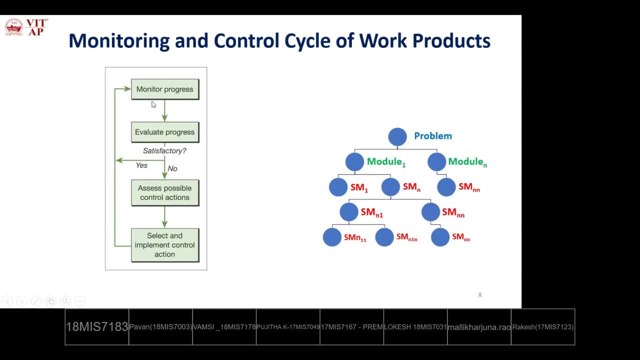 tasks, subtasks and so on. okay, so monitors the progress of all the project products, work products- okay, and then evaluate the progress. so what is happening here? evaluating, that is, whether we are finishing according to the schedule or not, or is there any delay in finishing the tasks? that we are checking? okay, so if there is any delay, 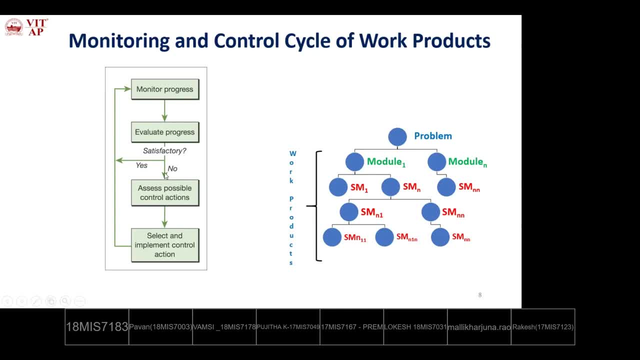 okay if there is any delay. so that is, some critical activities are existed. okay, so find the alternate solution, that is, a ss possible control actions. okay, and plan the alternate. so select and implement control action, plan and review with the other project products and repeats the whole process. okay, so whenever you evaluate the project product progress if anyone is satisfied, okay so 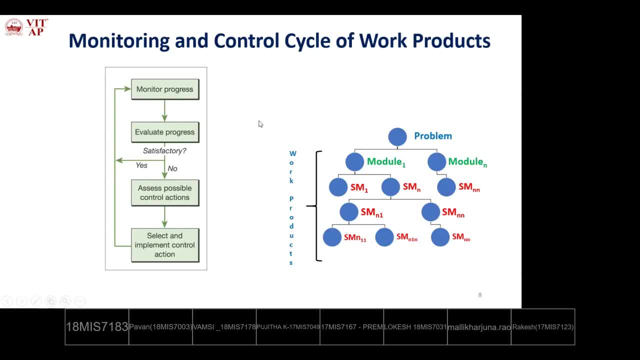 we'll integrate with the other modules. we'll integrate with the other modules and again we will evaluate, because when you will get the solution for this, whenever you find the solution for its next level, what are it? what are there in its next level modules. okay, every model is having sub modules. 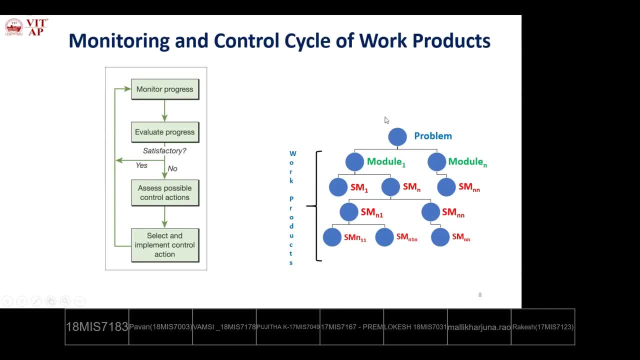 every sub models are having sub sub modules and so on. so here, in order to get the solution for this problem, we need to get the solution for this, we need to find a solution for this. okay, if you want get the solution for this, you need to find a solution for this. so what happens here? this model, 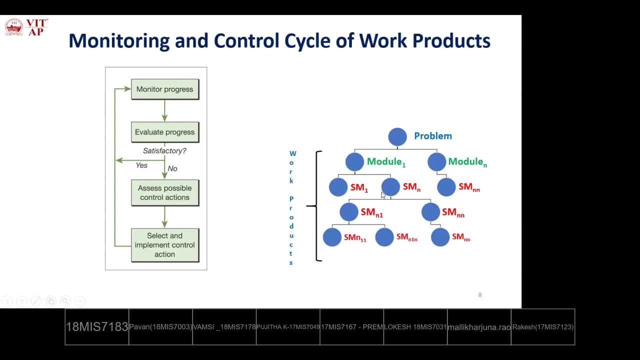 with the other modules. individually, every model may work, but whenever we integrate the one model with the other modules according to the dependencies are existed, sometimes my support may not support okay. so that's why we have to integrate with others and evaluate the progress of all the project products. when they works perfectly, then we'll find the solution for the final. 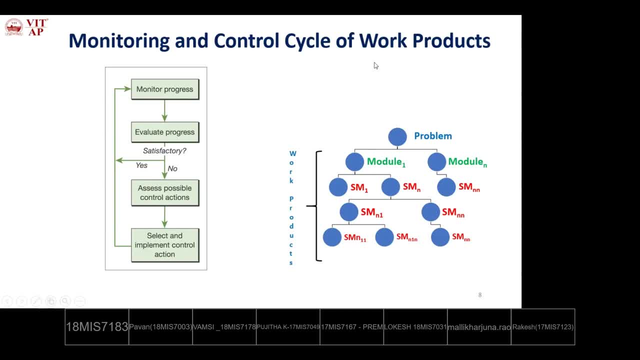 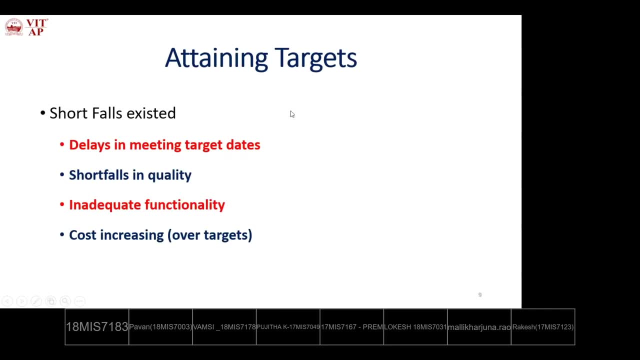 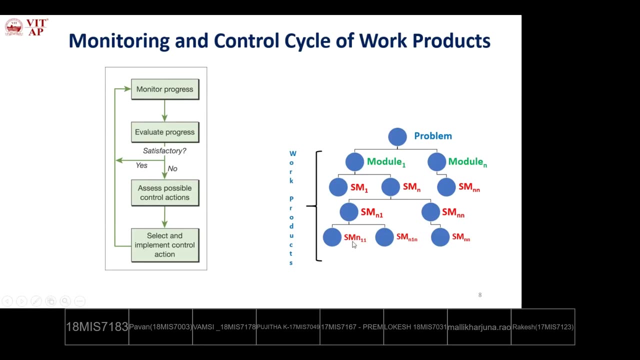 problem. okay, so this is a monitoring and control cycle of work products. then attaining targets, achieving the targets- what do you mean achieving the targets? so here i told you, every project product is having start date, end date. okay, so that we are checking here. okay, achieving the? 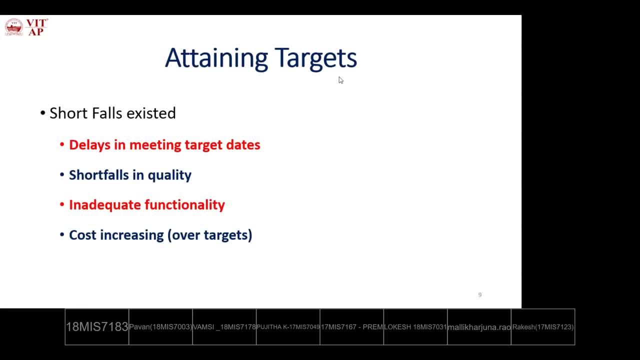 time. that is nothing, but are we working according to the schedule or not? is there any delay? if any delay is existed, how to overcome that? okay, so that is a. shortfalls are existed in the project development. okay, so in project development the various activities are not every activity is. 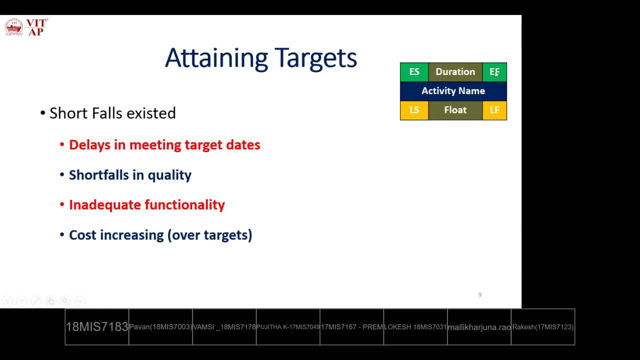 having a early start and earliest finish. okay, so this activity has to start by this time and finish by this time, by any chance. if any activity is delayed, what is the maximum way we can wait? that is the waiting period. this is the latest time to start. okay, if the activity is started by this time, what is the latest finish time? okay, this is the maximum. 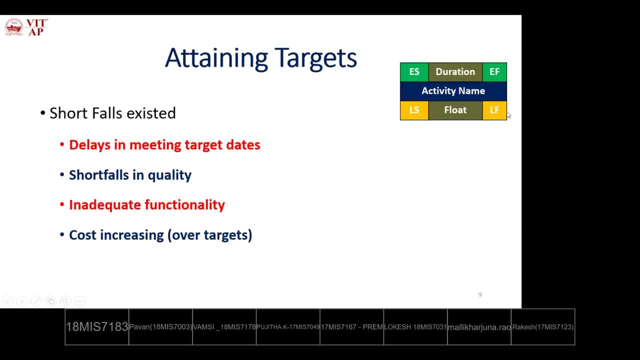 time that we can spend for on this activity, not the project on this activity. okay, so, yeah, so these these are happening generally when critical activities are existed. so if any critical activity is existent, then at the beginning of the activity the activities are not working. does not happen generally. 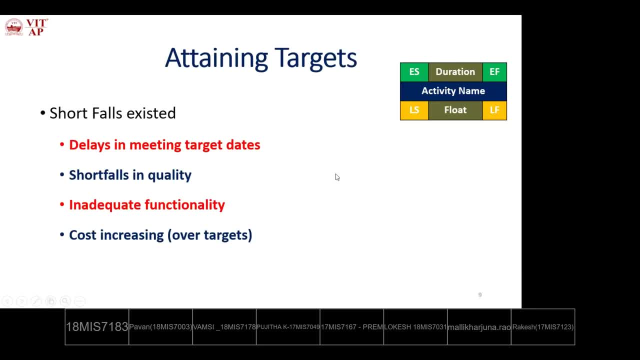 It's not easy to achieve the targets, So we are trying to finding those. okay, So shortfalls are existed, delays in meeting target dates. So why delays? Why delays are happening? Generally, the project is always getting delayed to deliver to the client because of changes. 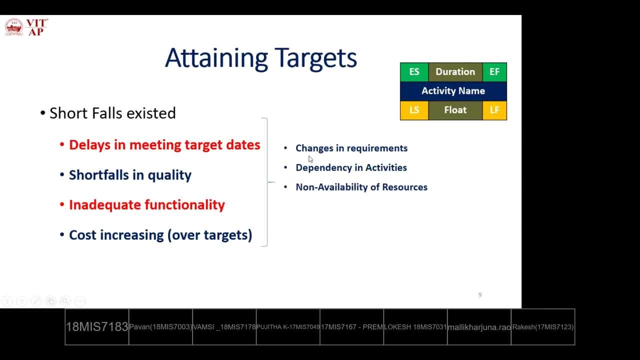 existed, Okay. Changes due to changes suggested by the client: okay. So we have to accommodate the changes, okay. Why? the greatest advantage of software is flexibility. software can support changes at any time during development, that is, from analysis to maintenance time. okay. 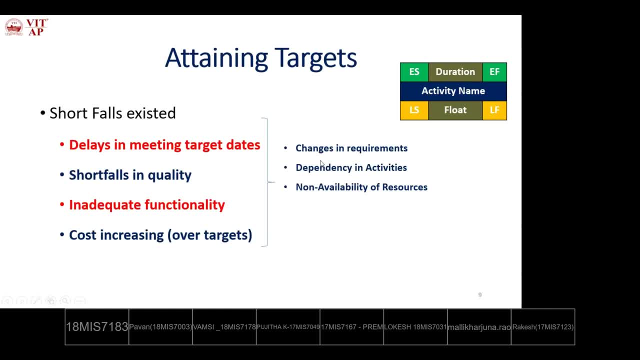 So we have to accommodate the changes as per the client need or demand. okay, So whenever you try to add the change, what happens? It shows the impact on the remaining depending activities, Not all the activities if it is having a link with other activities remaining depending. 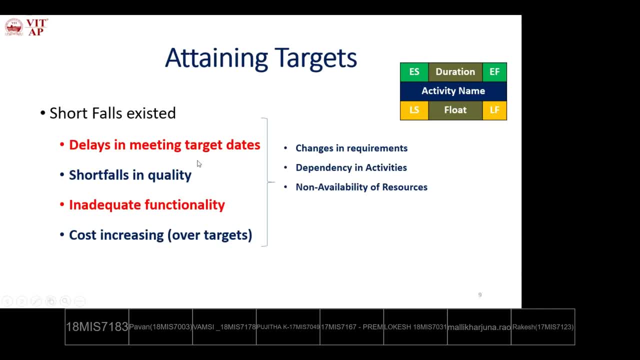 activities: okay. So delays in meeting target dates, then shortfalls in quality: okay. So when depending activities are existed in the software development, definitely quality is affected. Okay. So, for example, take the case Google products. what are various Google products? Gmail, YouTube. 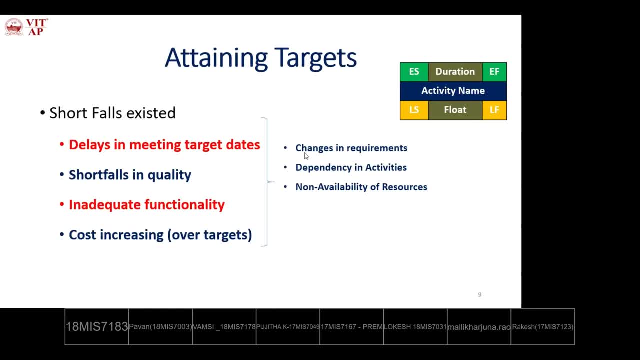 Google map, photos drive, et cetera, et cetera. So I you have one situation, that is, you want to send a large file to your friend. So what you will use, for example, anatomy file or 1GB file.